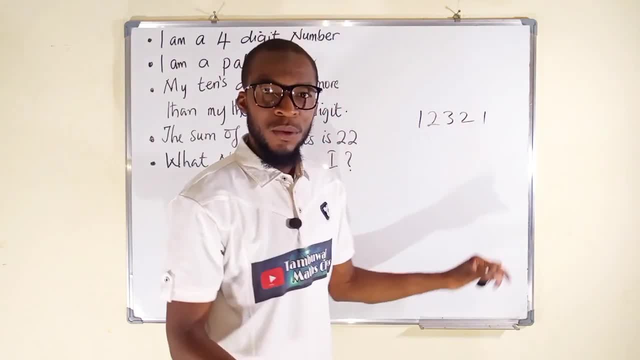 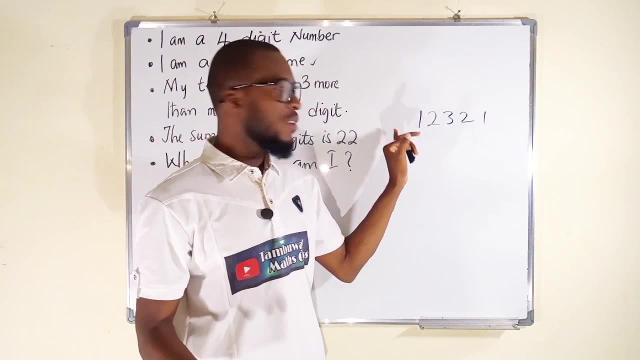 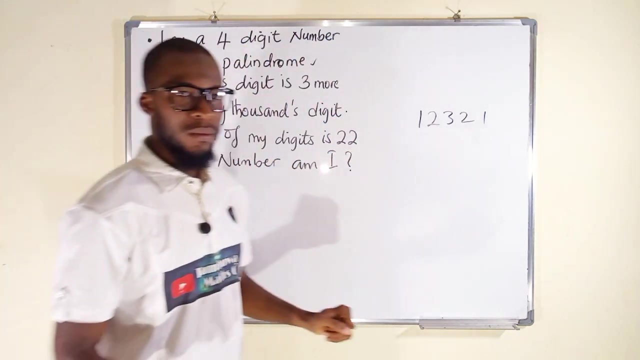 one, two, three, two, one. Look at this pattern: One, two, three, two, one. Backward: one, two, three, two, one. The way it reads forward is exactly the way it reads backward, But this question says I am a four digit number, So let's consider four digit number: One, two, two, one. Look at: 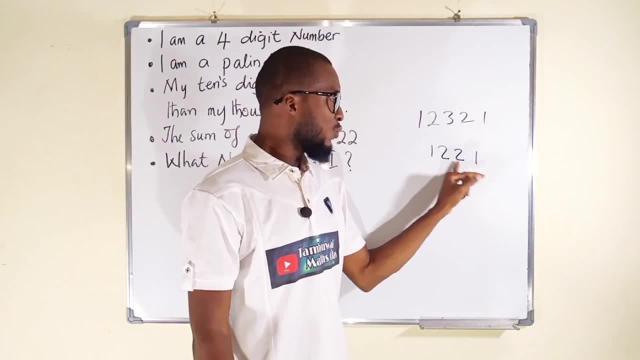 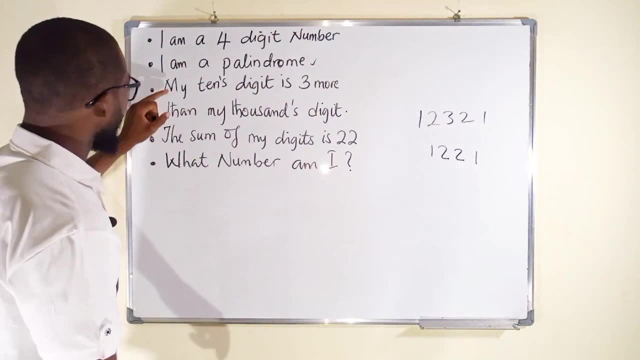 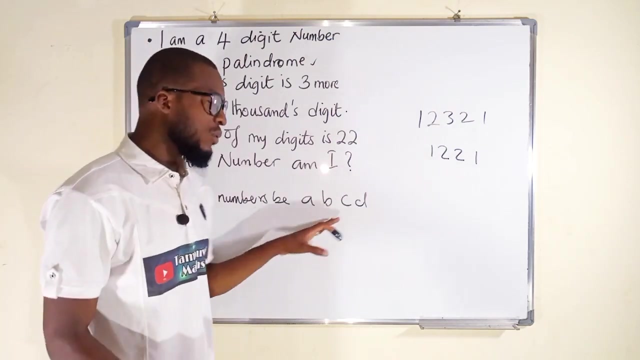 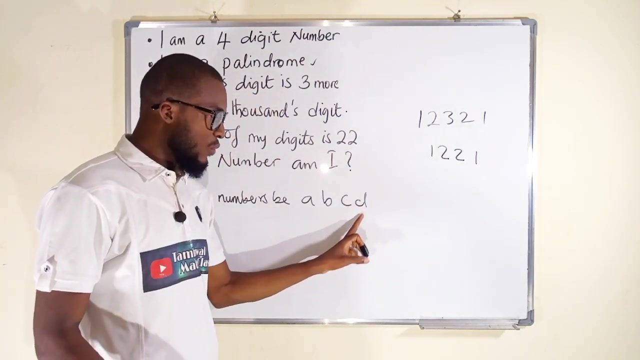 the pattern: One, two, two, one, One, two, two, one. The way it reads forward is exactly the way it reads backward. Okay, let's continue. So for this, let the numbers be let. We are going to find out these numbers later. My tens digit. What is tens? You know this is unit, tens, hundred. 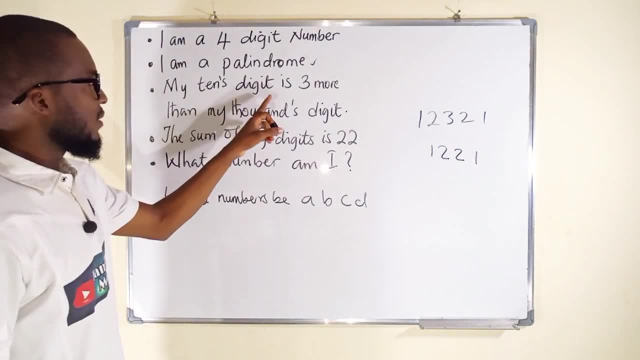 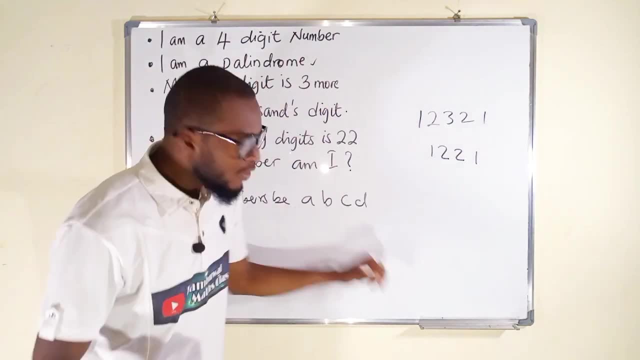 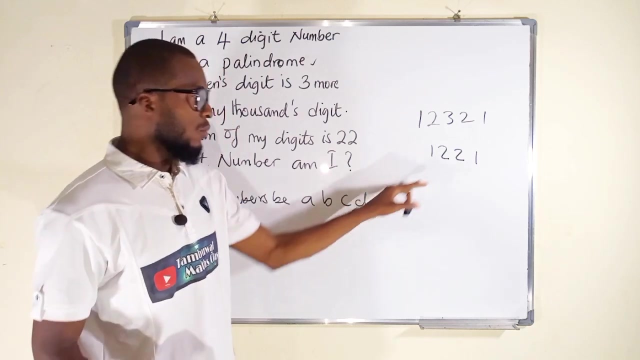 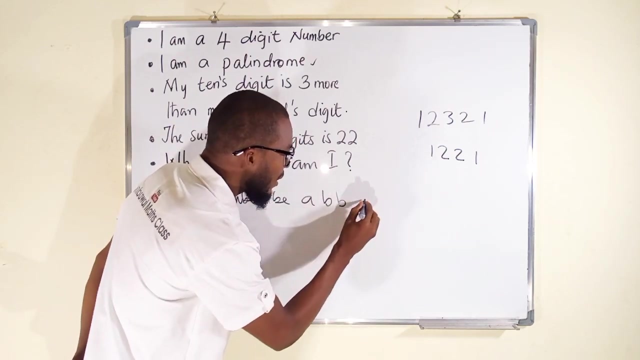 thousands. It's three more than my thousand digits. First of all, knowing that this is a palindrome, the first and the last digit must be the same. The second and the third digit must be the same, considering this pattern. So this must be B and this must be A, If at all we want. 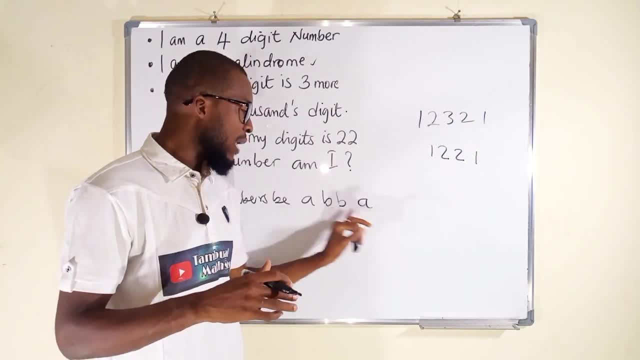 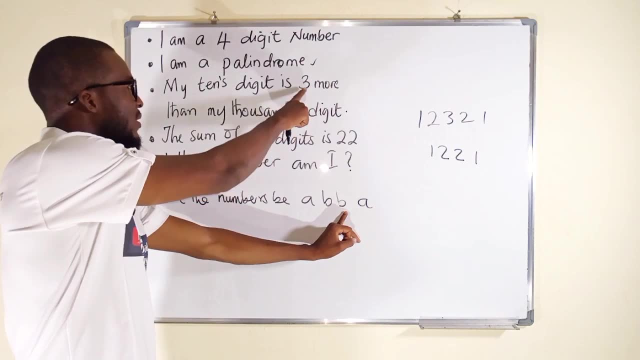 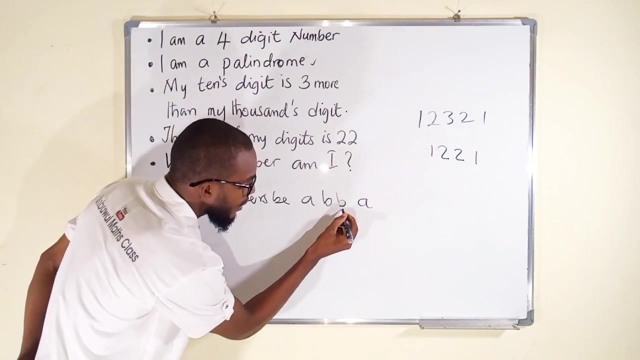 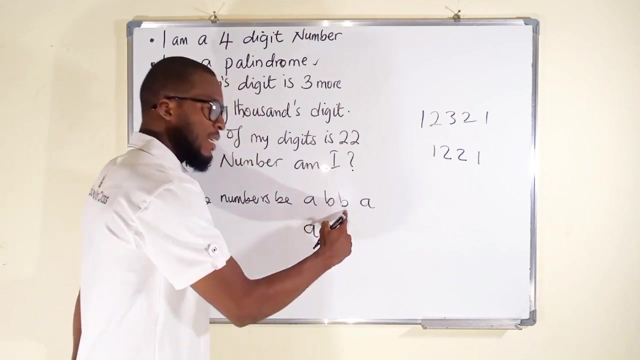 to consider it as palindrome: A, B, B, A, A, B, B, A. You get it. Okay, the tens number or the tens digit is three more than thousand digits. This is the thousand digits, So this number here is three more than this. So we have A, We have B. 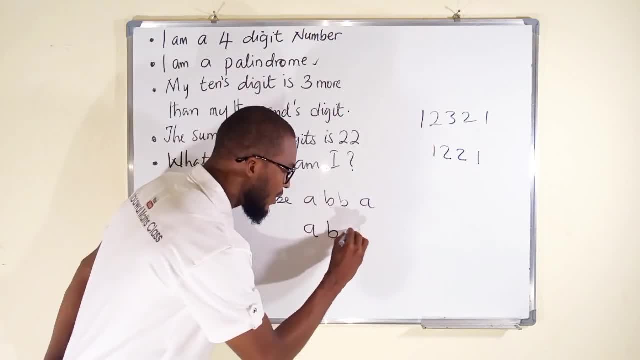 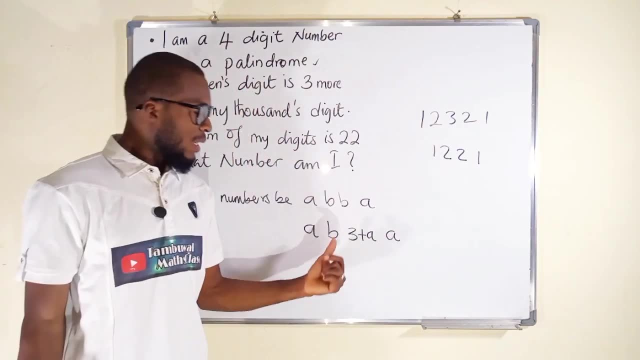 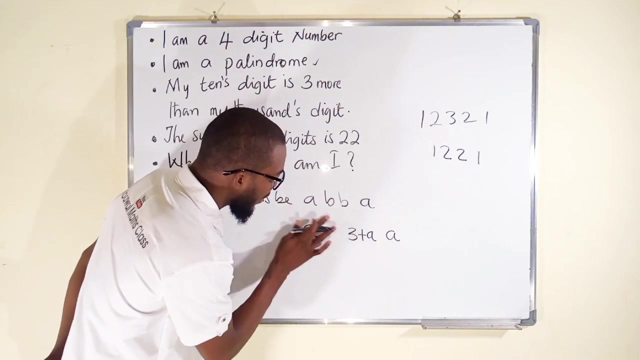 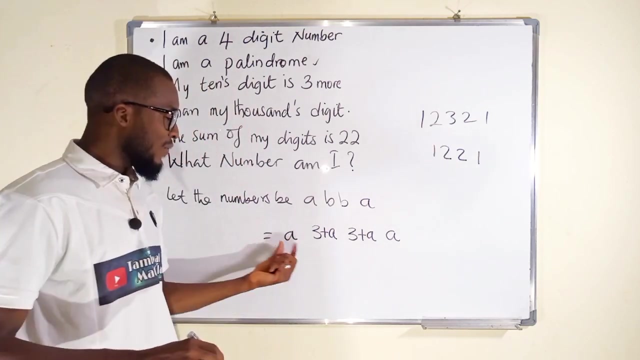 The tens digit is three more than this, So we have three plus A instead of B, And the last one is still A. But remember, the second and the third one must be the same. therefore, this must also be 3 plus a, so we can write this one as 3 plus a and we have our a here, so we have 3, 3 plus a, 3 plus a, a a 3. 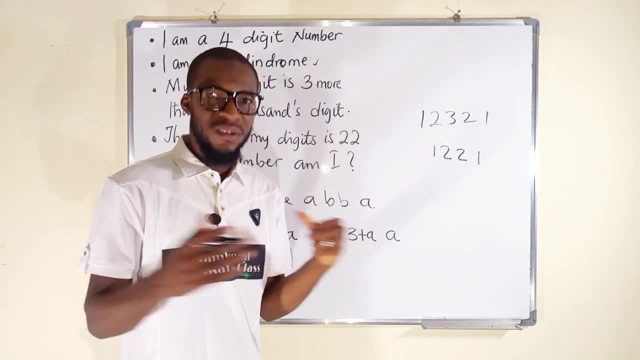 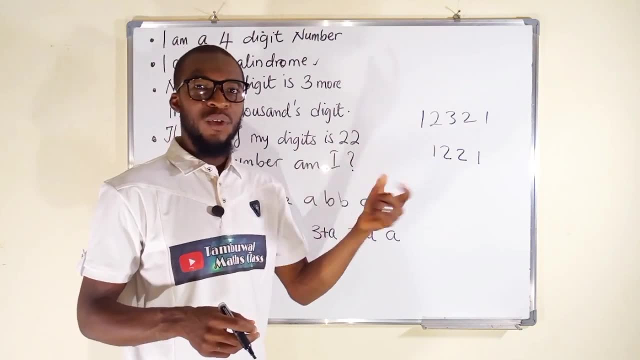 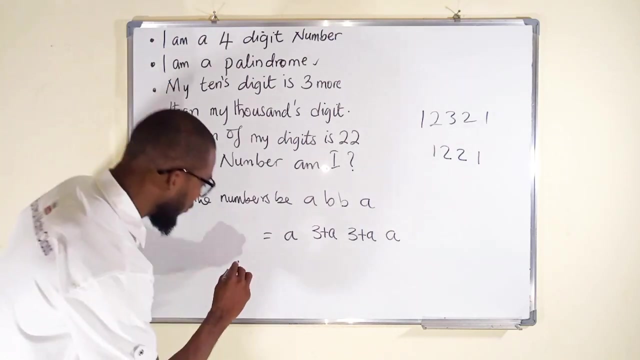 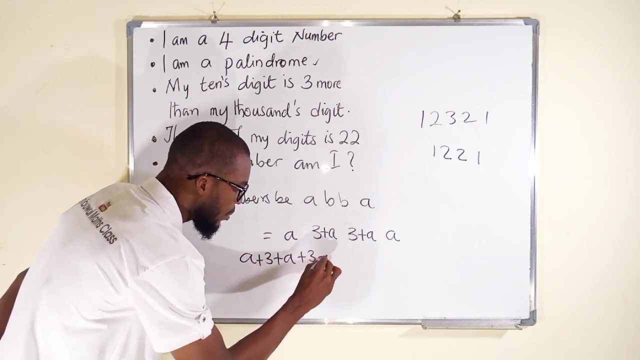 plus a, 3 plus a- a. in either way, it must reads the same way. let's continue. but it says that if you add all of these digits together, you're going to obtain 22. so we are going to add all of these digits and set them to be equal to 22. so we it means that a plus 3 plus a plus 3 plus a plus a. 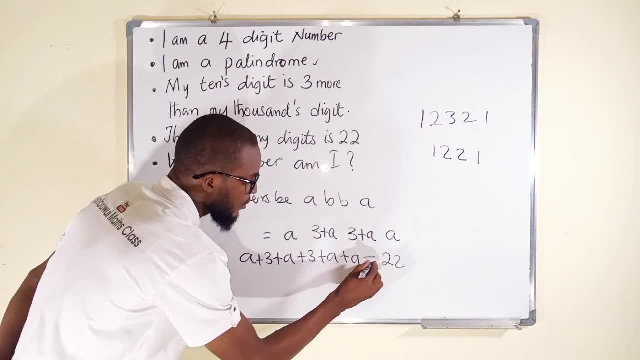 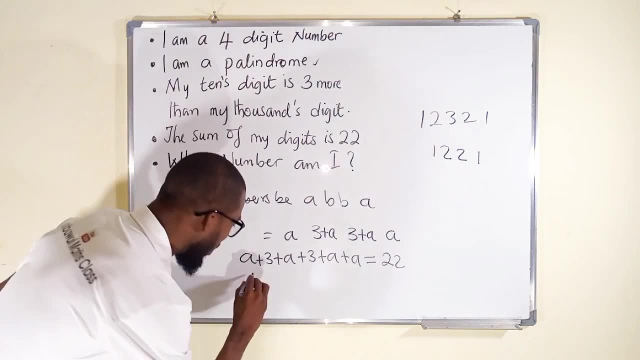 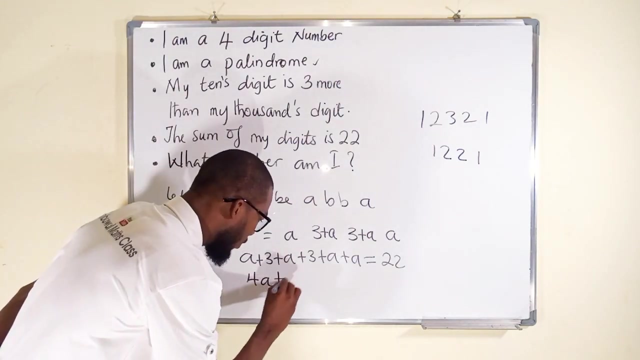 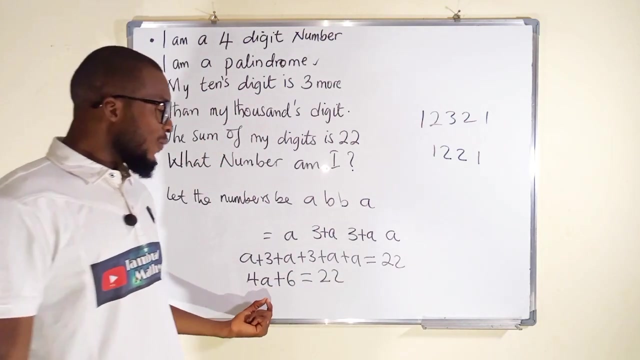 the whole of this must be equal to 22. according to the question, a, a, a a, there are four, so we have four a's three, three, there are two, we have six and this is equal to 22.. we are going to solve for a substituted back in this. 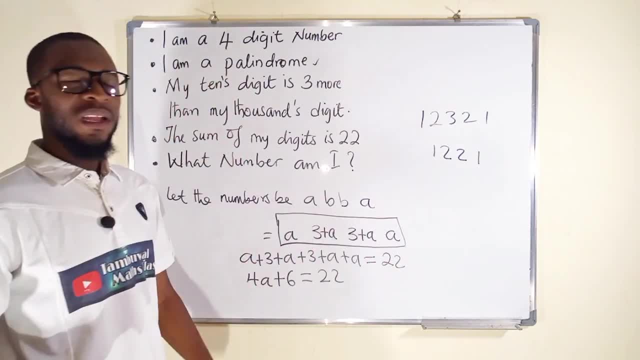 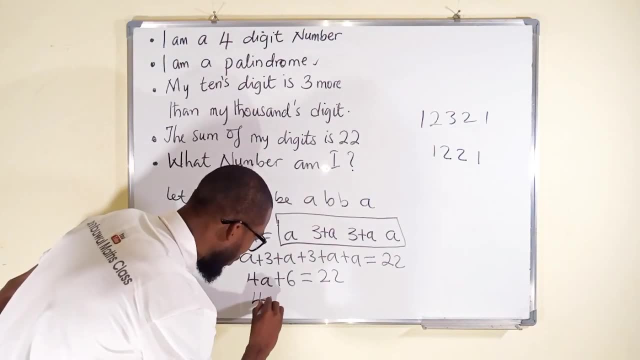 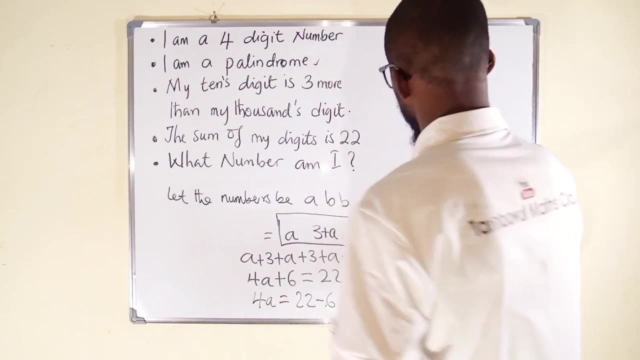 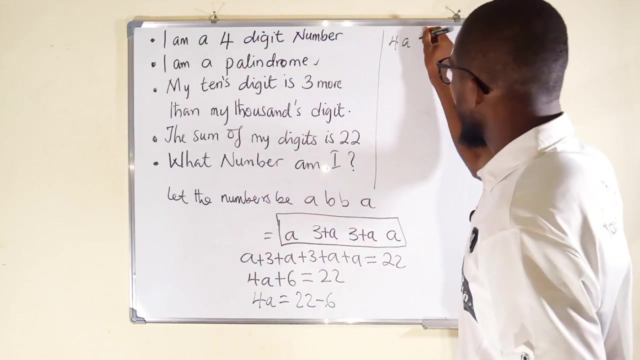 expression to obtain the required number. taking positive 6 to the right, it becomes negative. so we have 4 a equals 22 minus 6.. let me continue. the other side: 22 minus 6 is 16. we have 4a equals 16.. to find the value of a, we divide both side by the coefficient. 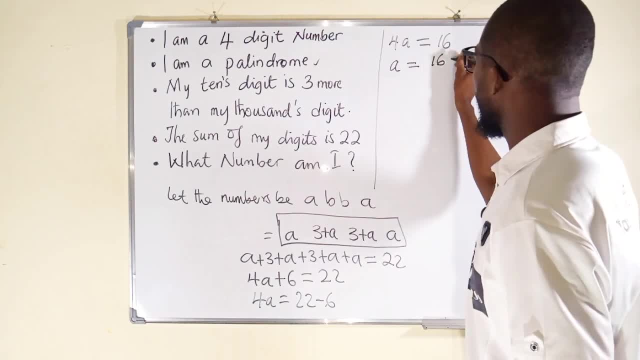 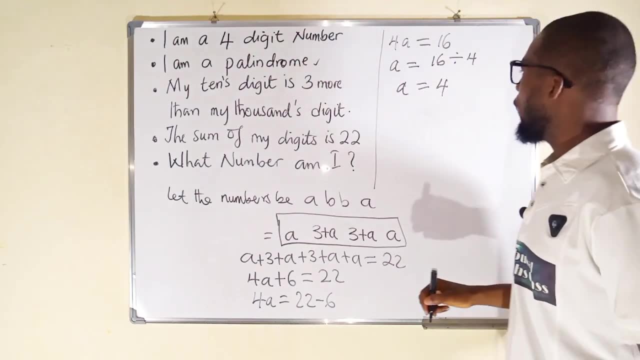 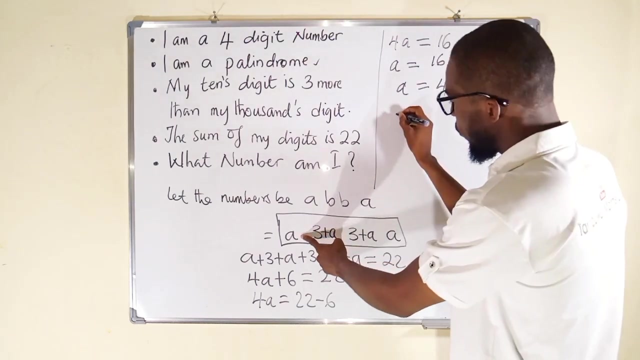 of a, which is 4, so we have a to be equal to 16 divided by 4. and finally, a is equal to 4, because 16 divided by 4 is 4. four, now let us substitute everything here. the first digit is a and a is four, so we have four. 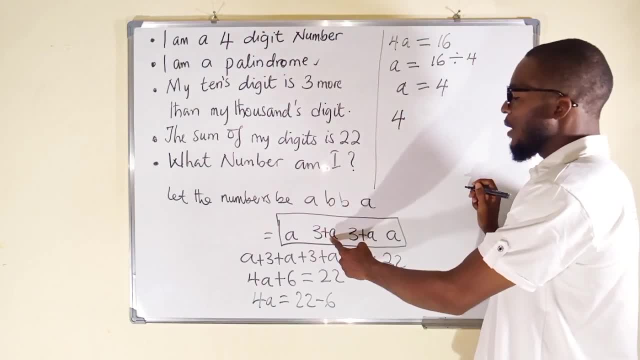 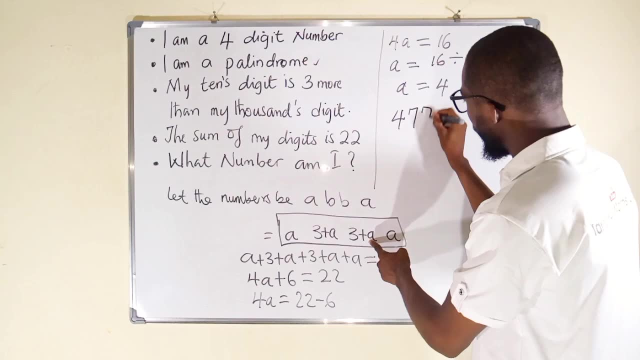 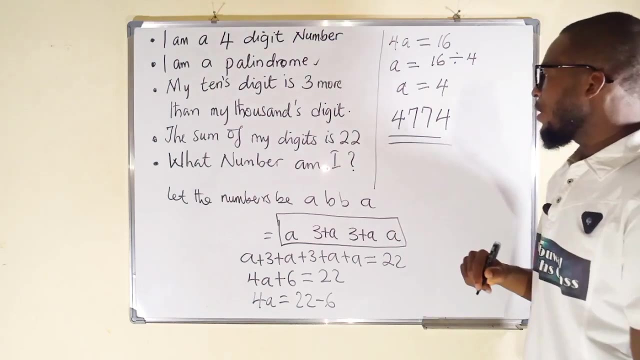 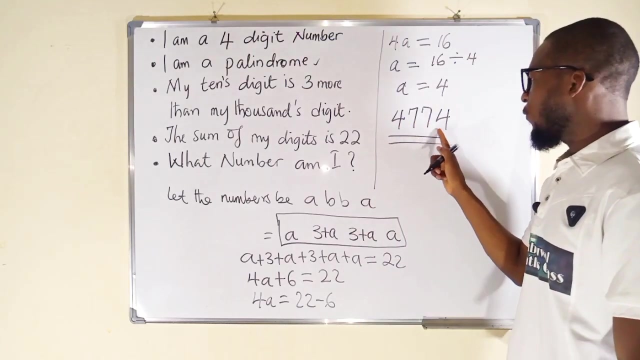 here the second digit is three plus a, meaning three plus four, which is seven. three plus four is also seven and a is four. therefore the digits, the required number, is four thousand seven hundred and seventy four. you can see the pattern in mendicant: four, seven, seven. 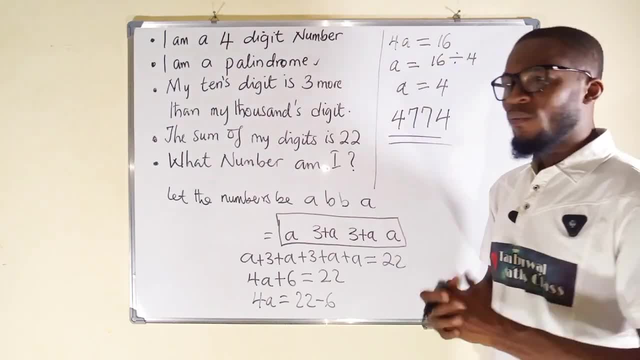 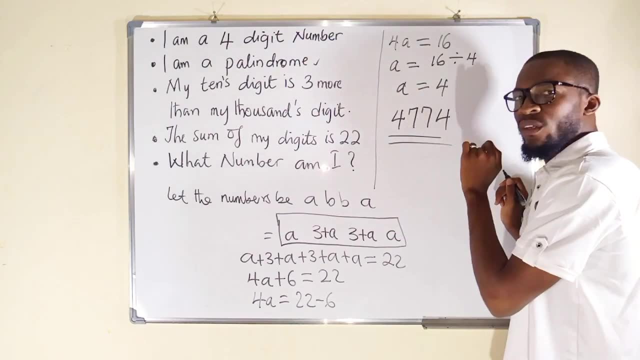 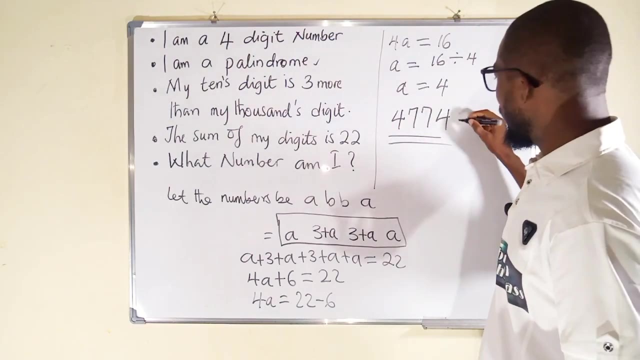 four, four, seven, seven, four, and let us add all of them together to see whether we're going to obtain 22 or not. remember that seven plus seven is fourteen, fourteen plus four is eighteen, then eighteen plus four is twenty two, and hence this is the solution to this problem: four, seven, seven. four. thank you for watching. Do have a nice day.